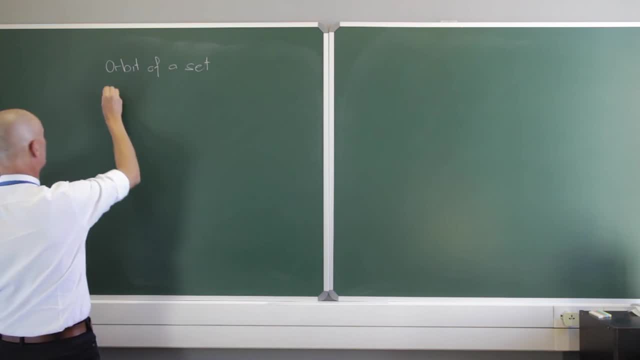 So we're going to imagine that we have two things. We're going to have a group G. It's going to have a set. I like writing that as G set these days. And some group action. 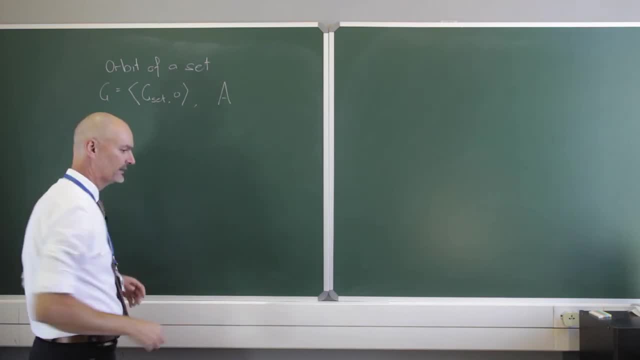 And we're going to have a set A, just a set of elements. And what we're going to take is we're going to take a specific A, which is an element of A. 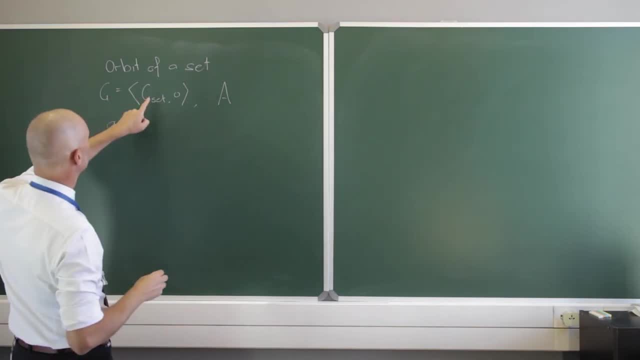 And we're going to allow all the elements in the set to act upon this A. So that's going to give us this thing called the orbit of A. The orbit of A. 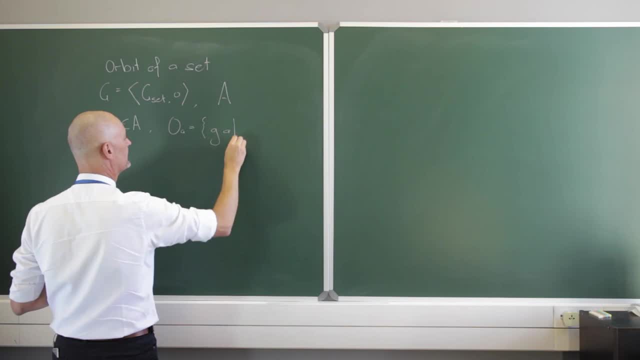 And that is a set G dot A such that G is an element. Of G set. 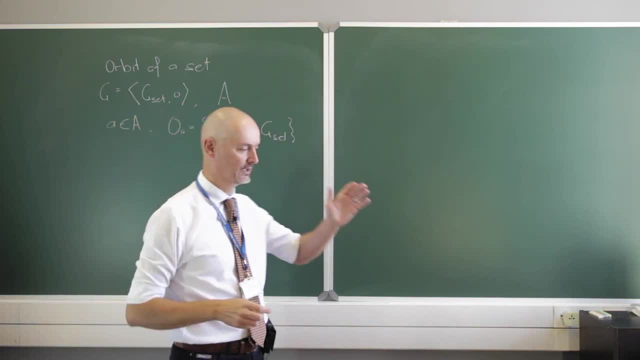 So what you can think of, you take all the elements of G, all of them, one after the other. You acted on this one specific A. 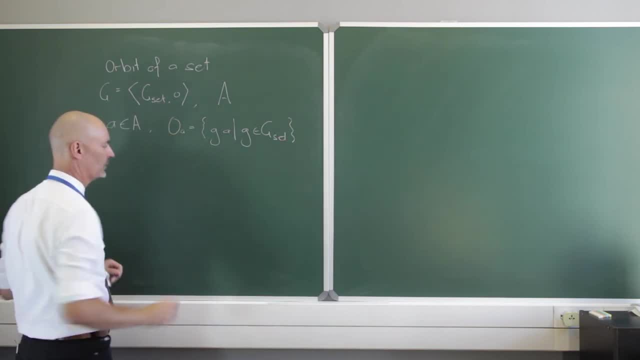 And that will give you a new set. And that set is called the orbit of A. 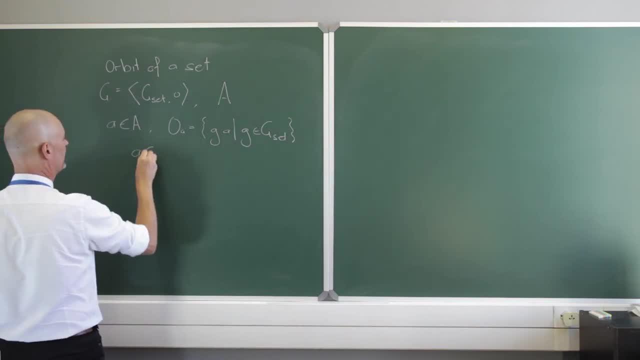 First thing that we'll notice is really that A is an element of the orbit of A. Why is that so? 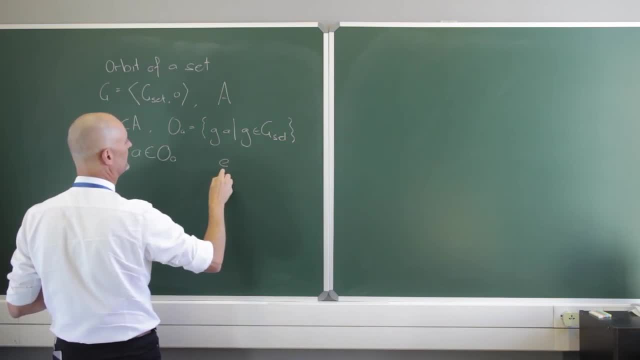 Well, we know that the identity element of the set G set. Is one of the elements in the set. 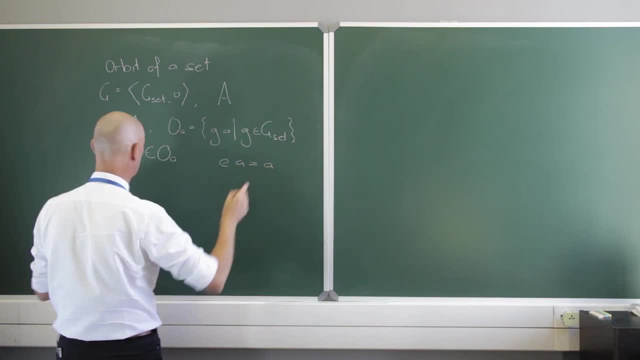 And if we act on A, we are just going to get A. So we know that A is an element. A is really an element of the set. So that is one thing we can look at. 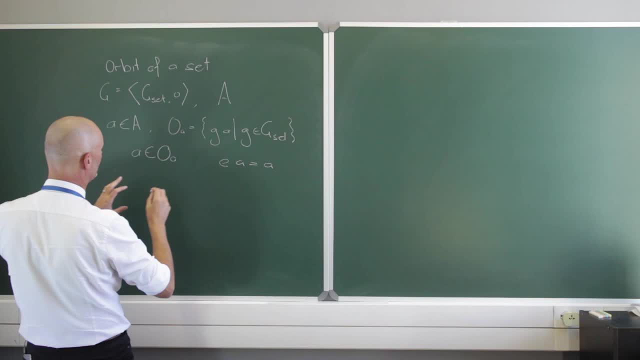 Just to see what goes inside of this set. The next thing we want to look at is if we take this set. All the G's acting on A. And. We take anyone, any arbitrary element of that. We've seen A is already in there. But we take any arbitrary element of that. Let's take G dot A. 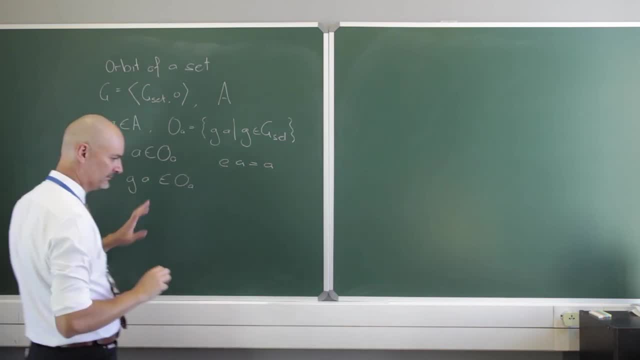 So that G dot A is an element of the orbit of A. As simple as that. 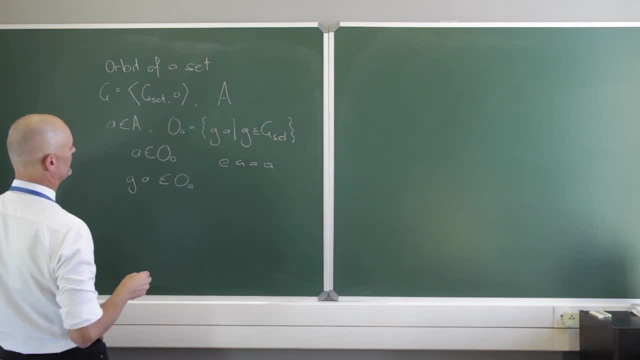 We just take any arbitrary one of them. What we are suggesting is that the set that we get from doing this. 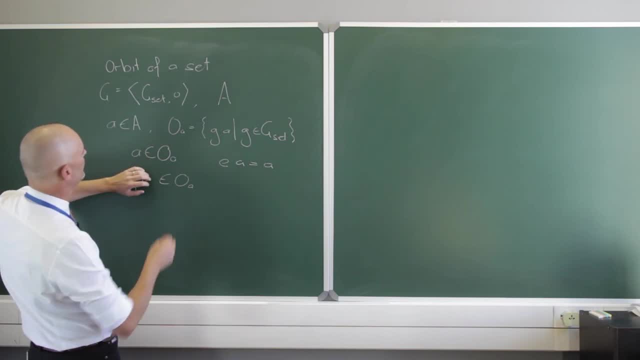 From taking one of these elements as our new element. As our new element. 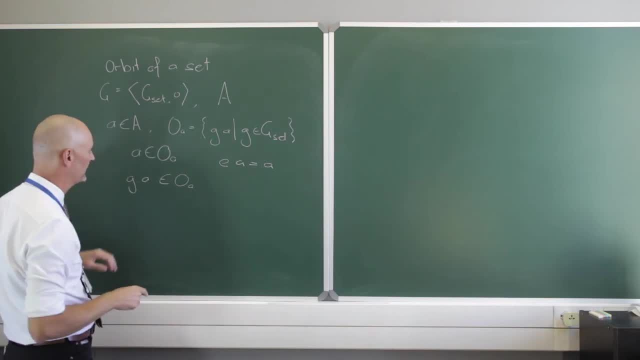 So we just take this as a new element of that orbit. That we are going to get exactly the same orbit back. We are going to get exactly the same. 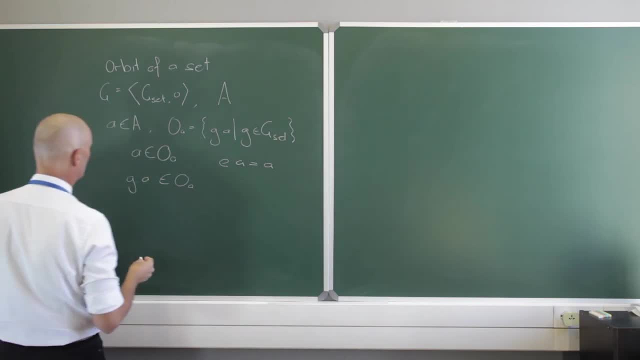 We are going to get exactly the same orbit back. And how do we know that? 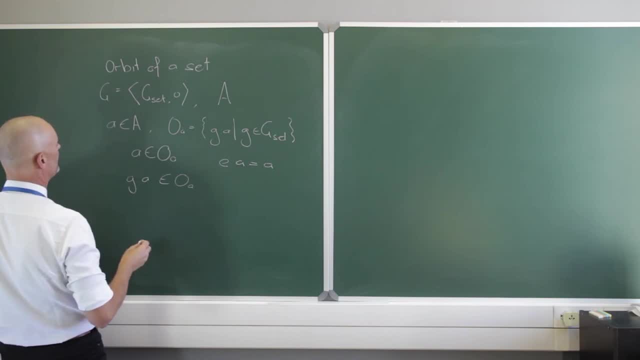 Well just imagine that we take G dot A. The, what we are, what we say the definition is. 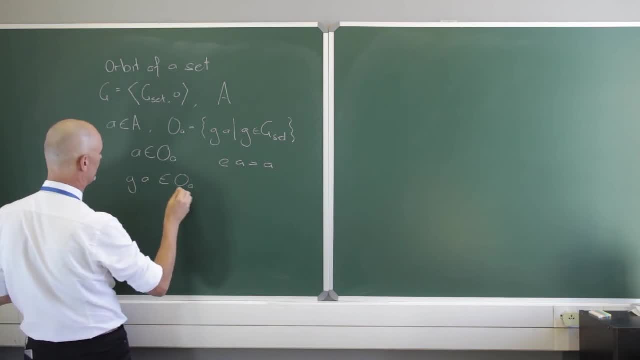 So now we are going to say that G A that is an element, let's call this of G A. So G A is an element. G A is an element of the orbit of G A. 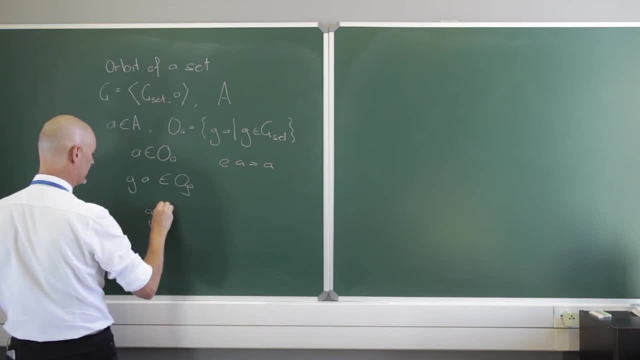 And let, what can we do? Let's take G star this time. And we act on G dot A. 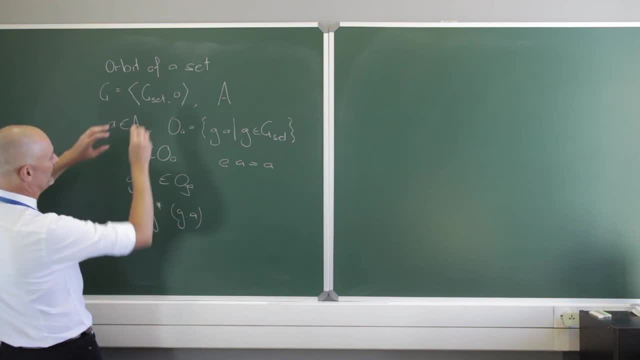 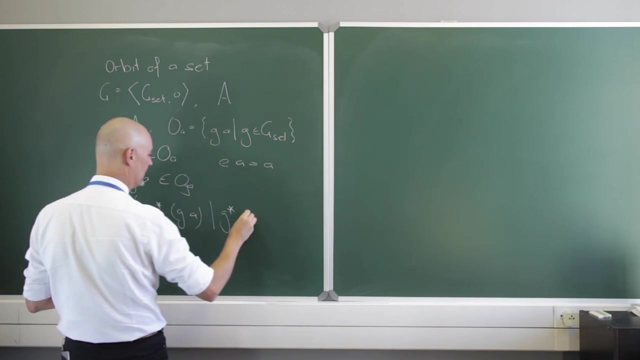 So what we are saying is this is exactly the same as our initial definition of the orbit of a set. We take all the elements G. So this is going to be a new set. And this time we just call it G star. Just to make sure that we are not talking necessarily about the same G. This is an element. This is an element of G set. In other words, we are going to run through again all the elements of G set. 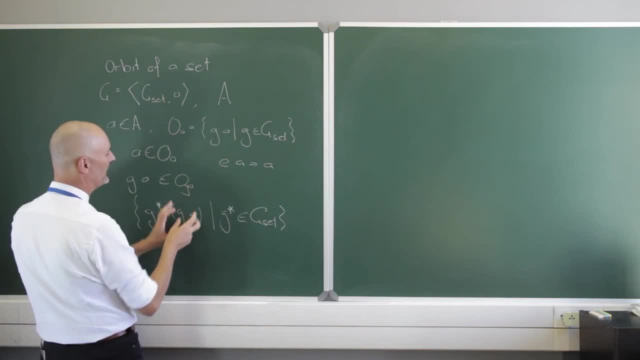 The set from my, and we are going to act upon this one element, arbitrary element that came originally from the orbit of A. So I should actually just say that. It is part of the orbit of A. Let's just do that, the orbit of A. And we are going to call this the orbit of G A. Because I am taking a new element. I am taking a new element. And remember that element is just another element of my set here. And I am doing this whole orbit thing again. 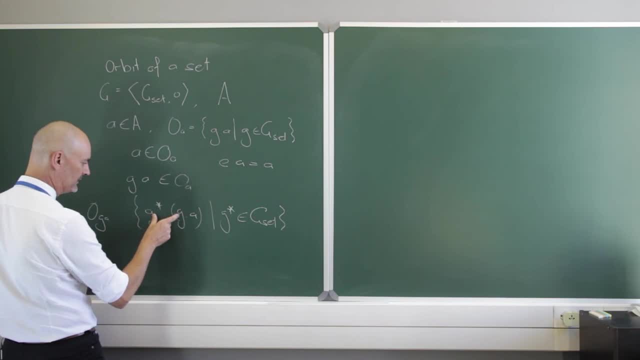 Now by the properties of group action, I can rewrite this as G star. And composed with G. That is the binary operation of that. Acting on A. That is what I can do. But by the properties of a group, this is just another element of G. This is just another element of G. So this, writing this, is nothing other than just rewriting this. Because I am taking all the elements of G and I am running all of them. And I am acting on A. All of them. 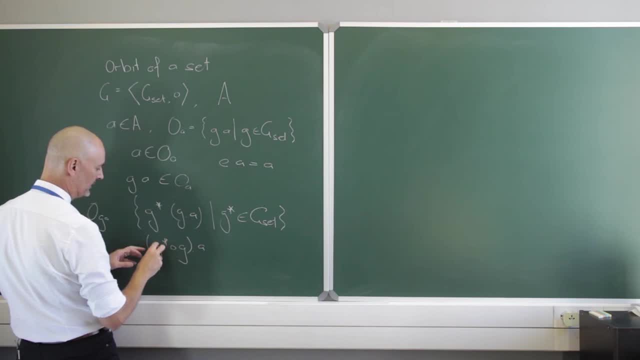 And I am acting on A. Because this is just under the column of G in my Cayley's table of group operations. 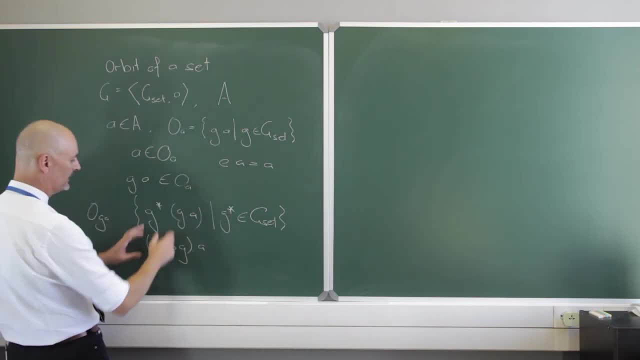 So by Cayley's theorem, I am just running through all of those again. So I am running through all of those, acting on A. Running through all of G set. G set acting on A. And this is exactly, so this is OGA. 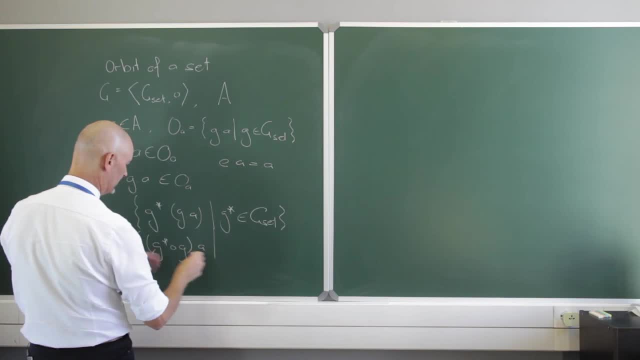 Is this, the set such that this, this is all elements of G set. 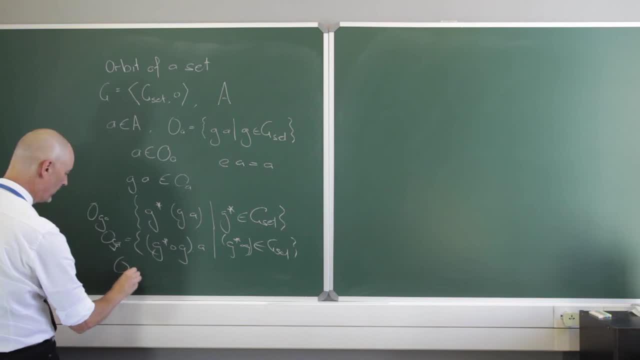 So I am running through all of them again. And what am I left with? I am left with the orbit of A. 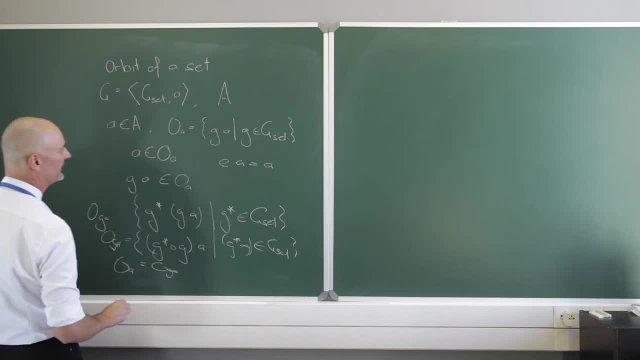 Because that is exactly the same thing. So those are exactly the same thing. So I can take, from the start, take an element of A. All the elements of G set act on that. That gives me a new set. 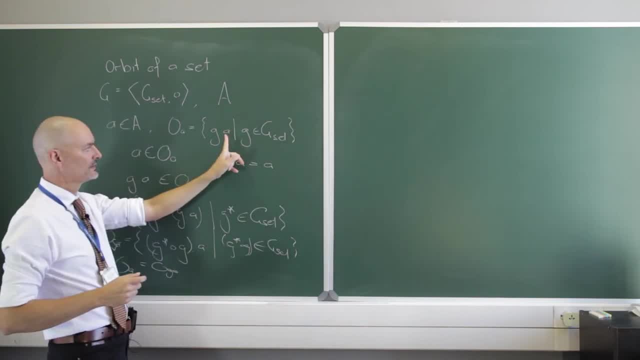 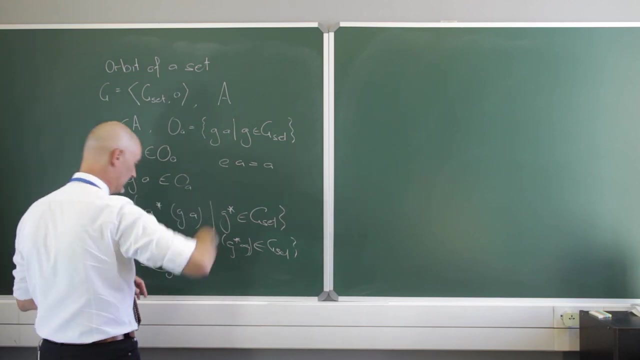 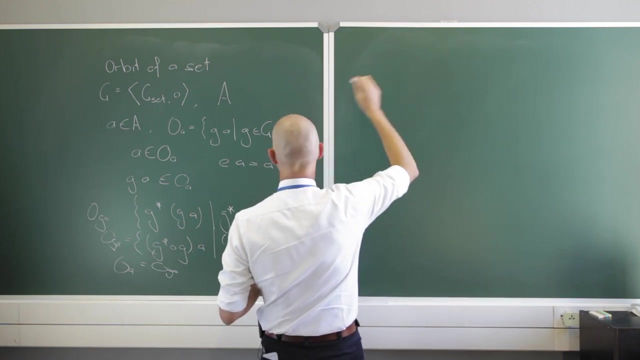 And I am saying this specific set. Which is very unique because it comes from A. Is I am going to create a set and I can take any one of those as a new element. I am going to take then a new, it as a new element. And I am going to let G, all the elements of G act on all of them again. And I am going to land up with exactly the same orbit. I am going to end up with exactly the same orbit. So that is very interesting. The other thing that we really need to note is the fact that, that this orbit of A is a partition. 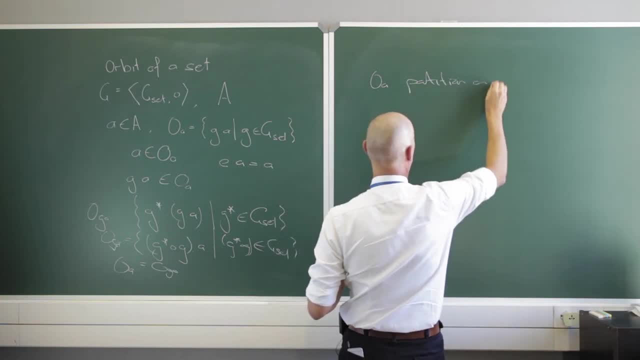 It is a partition on A. 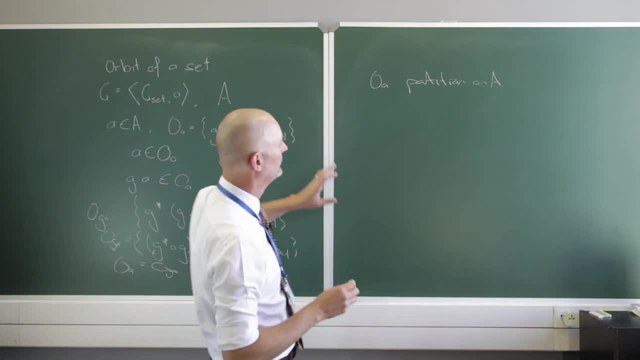 So it takes A and it partitions it. Well, what it might do is it might just be equal to A. That is just a trivial one. 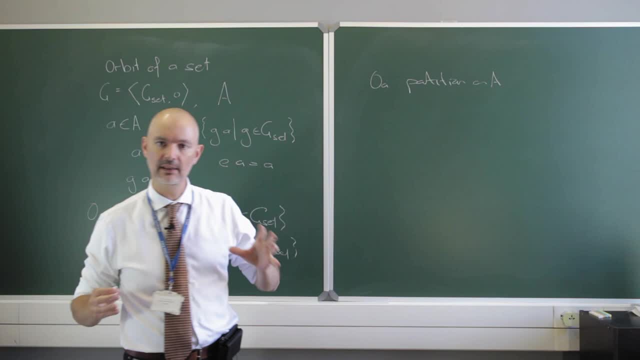 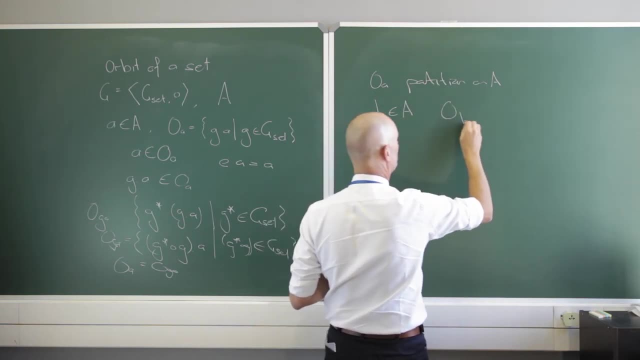 But let us imagine that it is not trivial and that there is another specific orbit. And we are going to take an element B. Element of A. So that we create the orbit of B. Remember that is going to be G dot B. And we run through all the elements of G set. 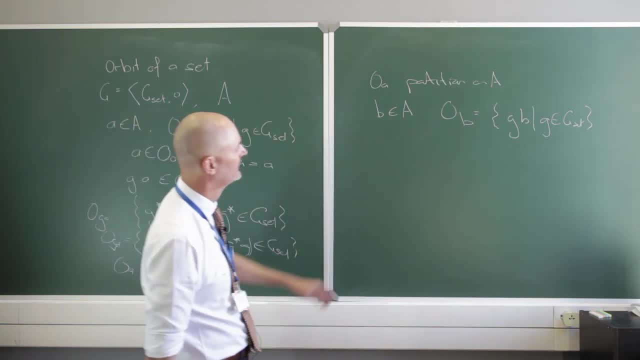 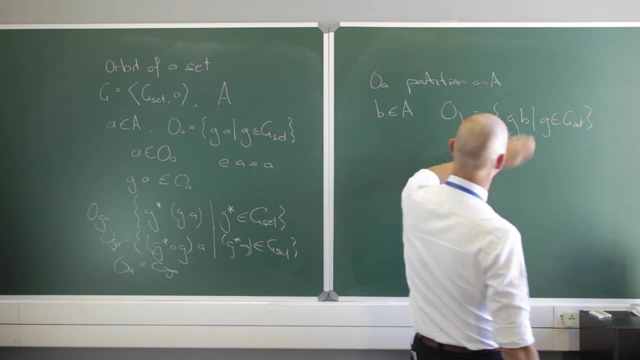 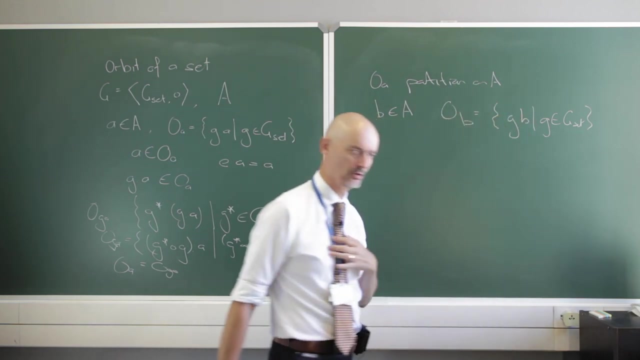 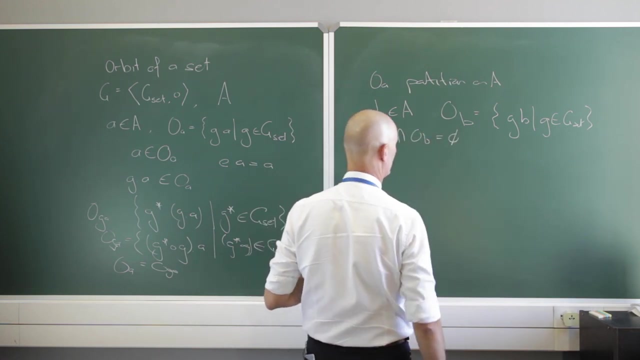 And what we are suggesting is that we can have these two be disjoint. So that if I have this element here. And it is, it is not part of that. You know if we can show that then it is disjoint. So that we have this, that OA, the intersection with OB. That that is an empty set. They are disjoint. 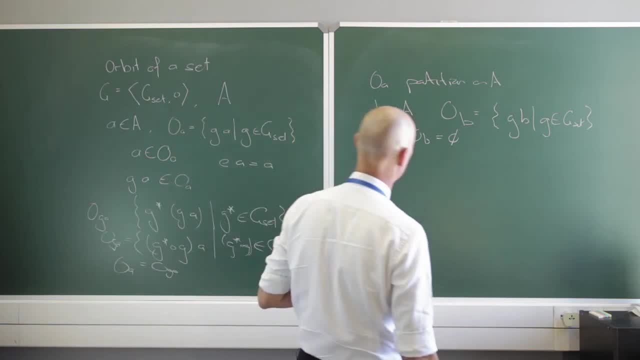 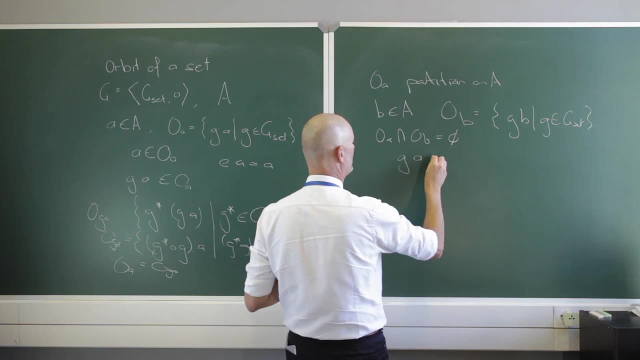 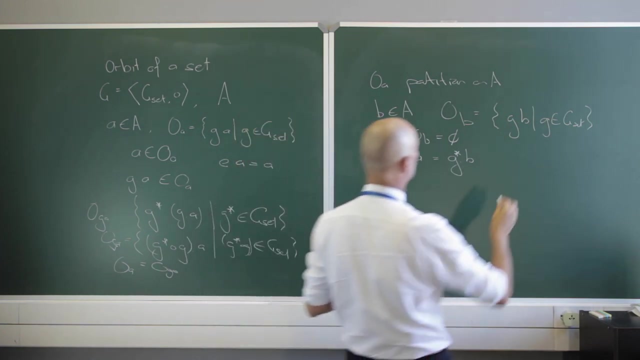 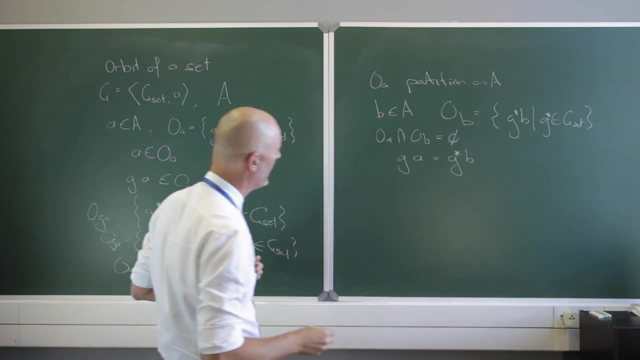 How would we prove that? How would we prove that? Now let us just to the contrary have this G dot A. And we set that equal to G dot B. And we are going to make this G star. Let us make this G star so that we know. And it is not necessarily that we start off with the same element. It is just we run through, we run through all of them. So let us say they are not disjoint. 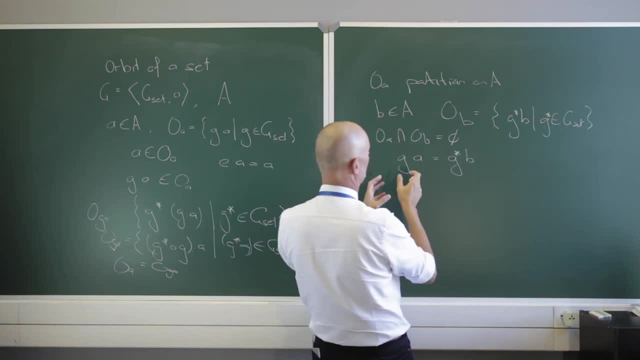 So that you know that these two. I can find an element in the orbit of A. 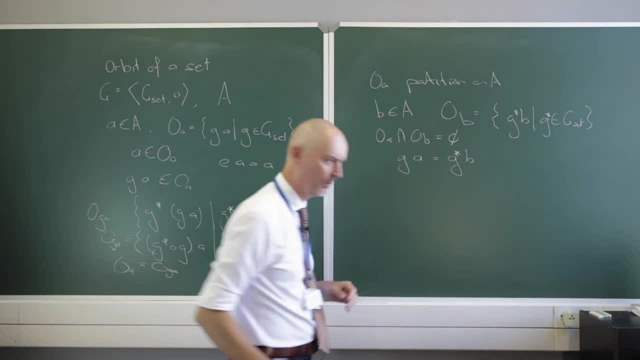 And that is going to be equal to some element in the G. In the orbit of B. Imagine then that that would mean that they are not. They are not disjoint. 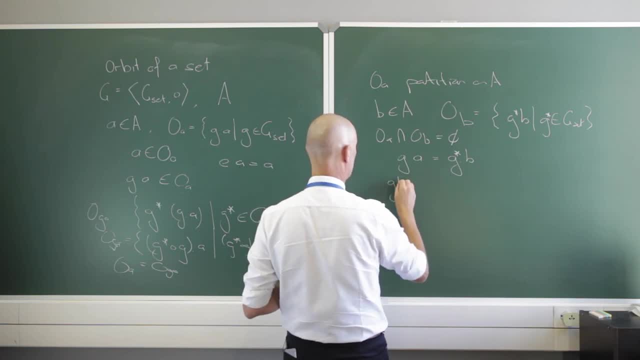 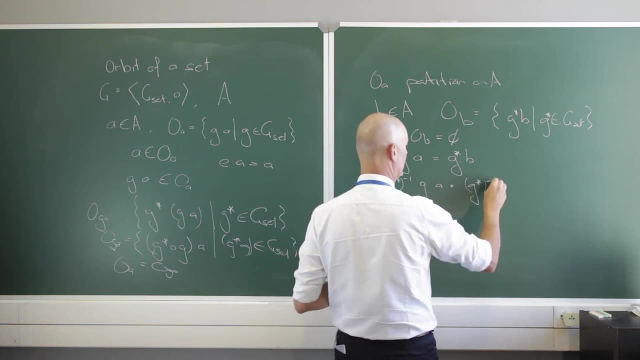 But let us act on the left hand side by G star's inverse. G dot A. And it is completely legitimate to do. 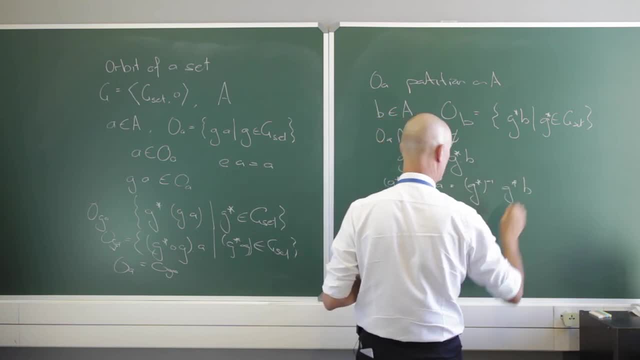 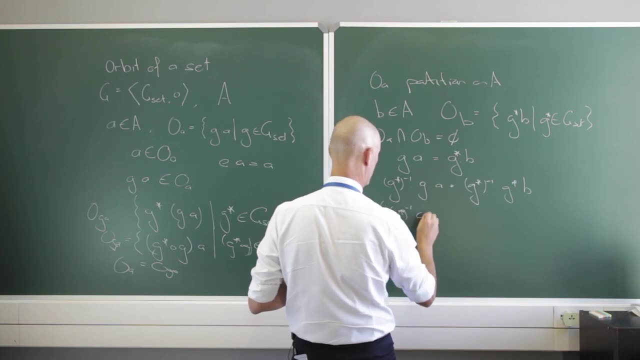 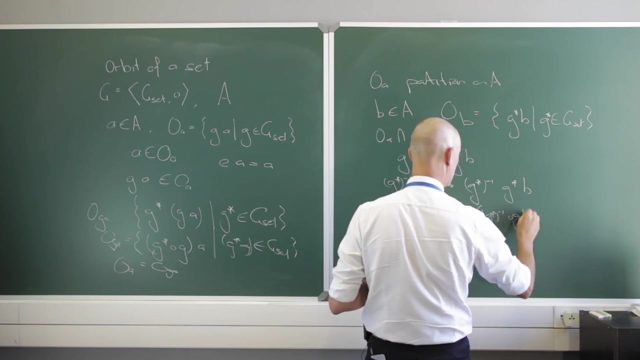 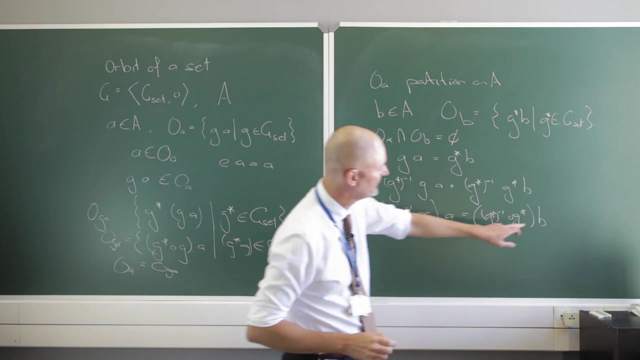 And I am going to G star dot B. By the properties you know what we can do. So this is going to be G star's inverse. Composed with G dot A. And this is going to be G star's inverse. Composed with G star. And that acts on B. We know from the properties of the group. That that would be the identity element. So we just have B on this side. And what do we have on this side? 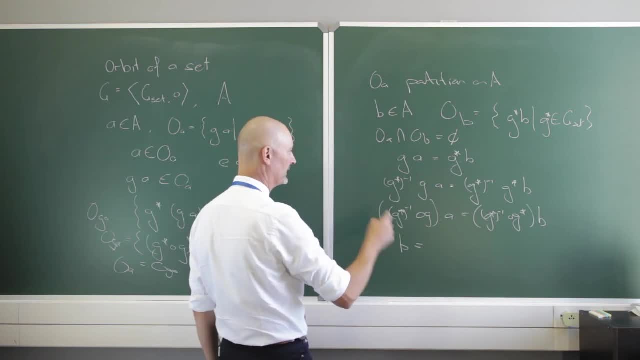 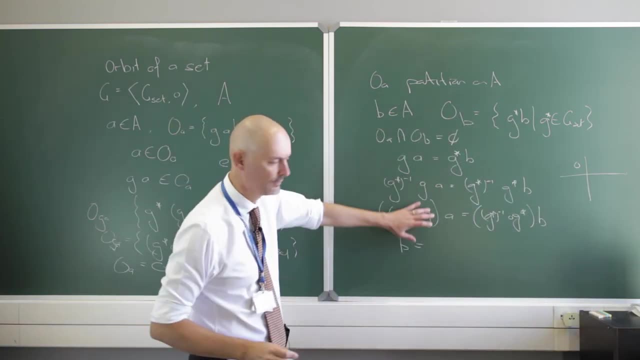 Well we are just running through all the elements. By the Cayley's table. For G. We are just running through a whole one. By Cayley's theorem. That means I am running through all of them. And what do I have? I have nothing other than G dot A here. 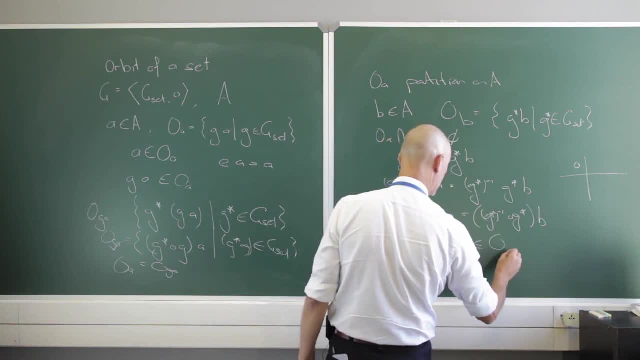 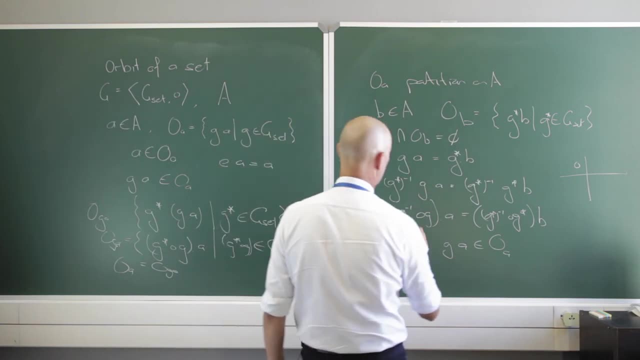 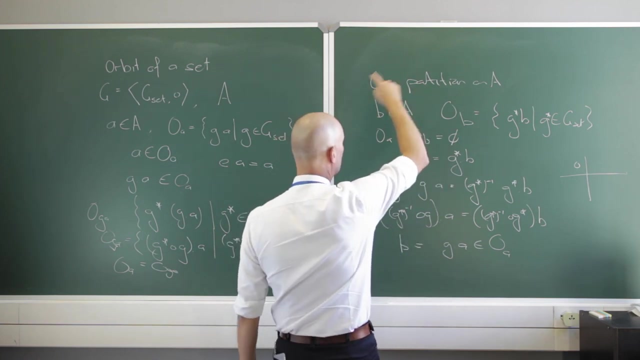 G dot A element of the orbit of A. So now B is an element of the orbit of A. So if this was so. Then it means it is originally part of this orbit of A. It is originally part of this orbit of A. 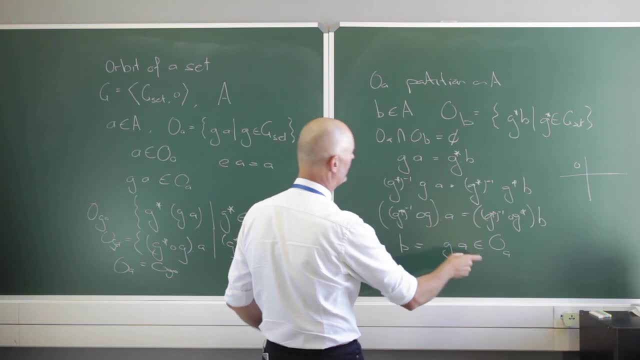 Showing that if it is not part of the orbit of A. Then we have two disjoint. Then they are disjoint. 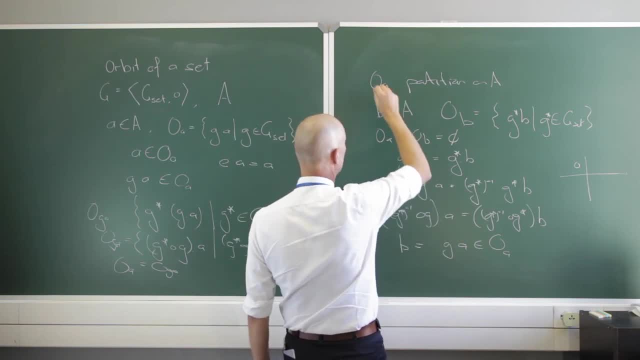 Showing clearly that if I do create an orbit. Say it is part of. 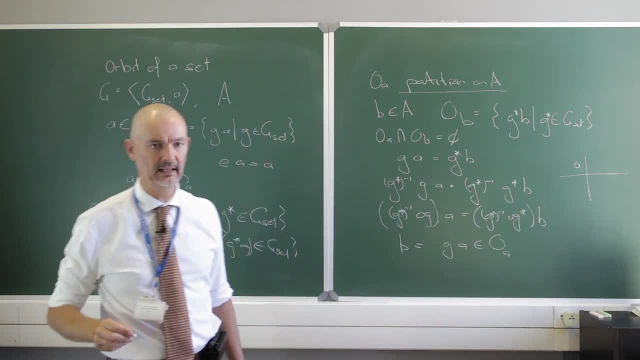 It is one of the partitions of my set A. 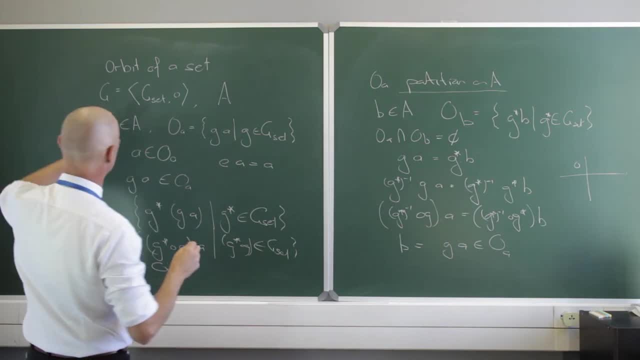 So in summary. A couple of beautiful things. We know the definition of an orbit. We take a specific one. We know that A itself will be an element of that orbit. We also know that if I take any one of the elements in that orbit. And I try to create a new orbit through that. 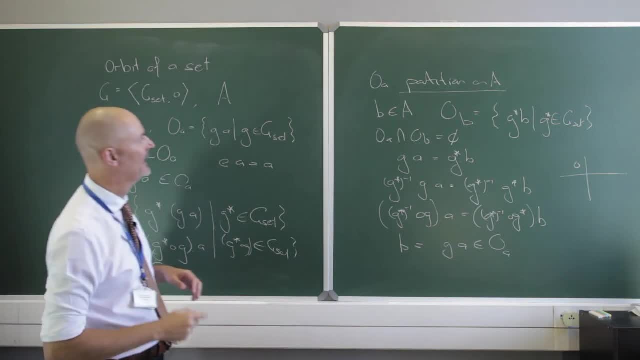 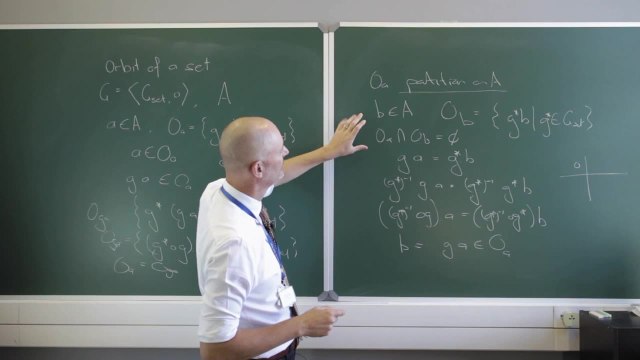 It is just going to be exactly the same as the original orbit. And that these orbits. They really partition. They partition a set. They partition the set. In these disjoint. In these disjoint sets. So that is the orbit. 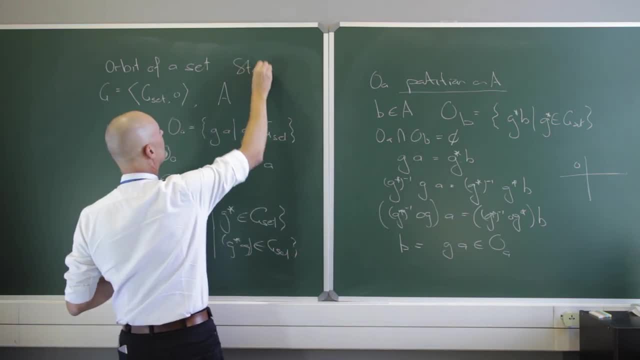 In the next video we are going to look at what the stabilizer is. 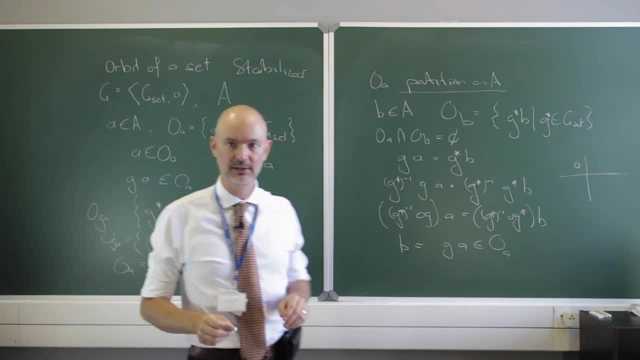 The stabilizer. And that is for the next video. 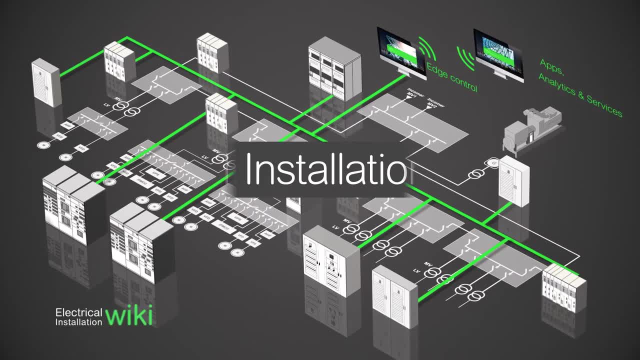 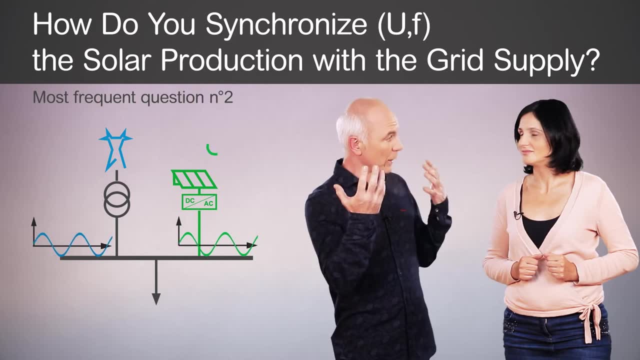 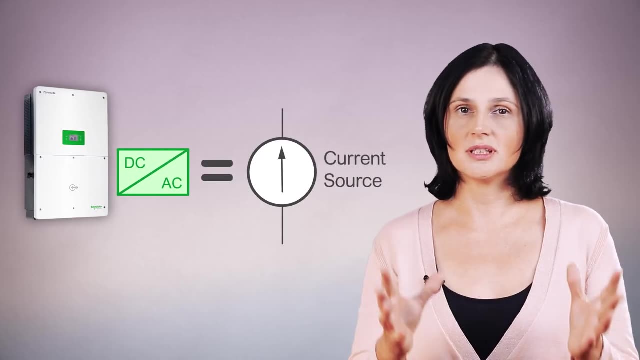 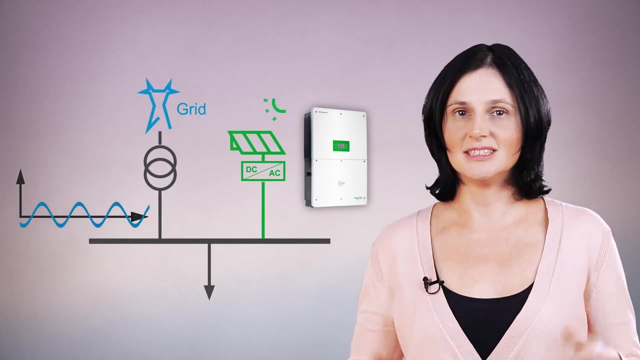 How do you synchronize the photovoltaic production with the grid supply? Grid-type photovoltaic inverters are current sources. They do not provide voltage and frequency reference by themselves. When connected to the electrical installation, they measure the voltage and frequency at their connection point and deliver a power output synchronized.